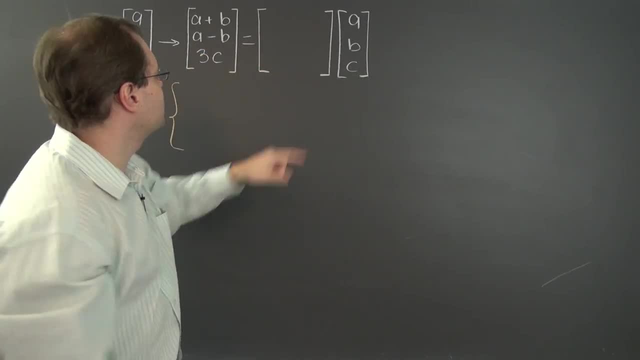 1, minus 1, 0, and 0, 0, 3.. So we have 1, 1, 0.. 1, minus 1, 0. And 0, 0, 3.. 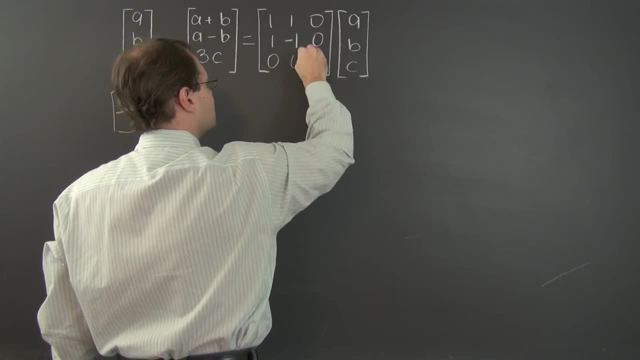 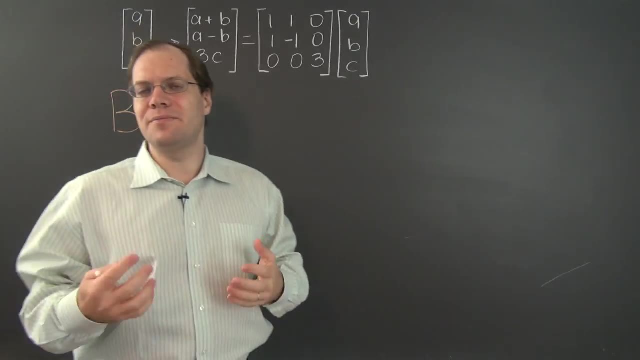 And this is a potential source of confusion. Of course, if you think about the length of the matrix, you can get an answer to that particular question. Okay, let's see what the answer to that question is. So, Of course, if you think about it carefully, there is no confusion, but it's important to realize that this is not a matrix. 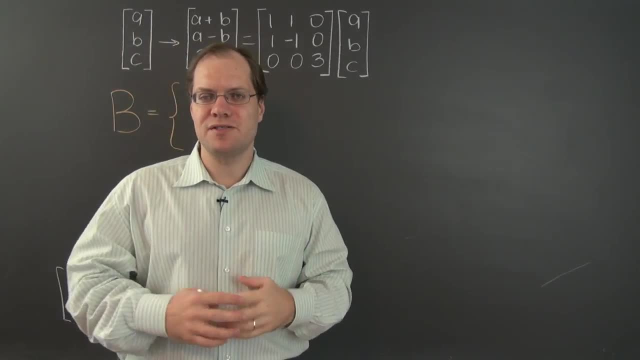 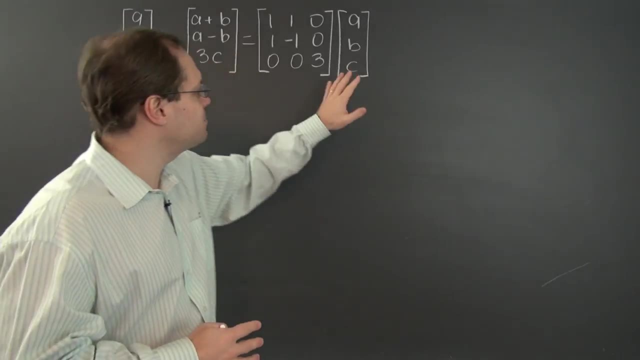 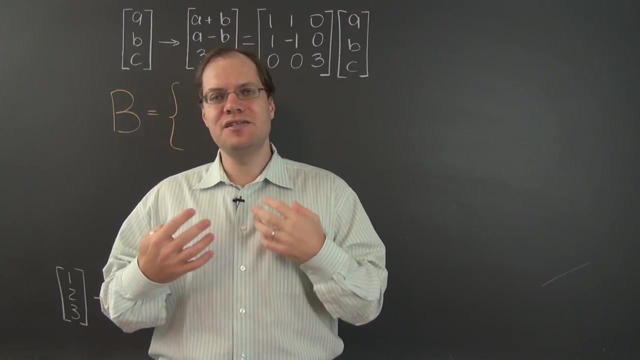 Representing this linear transformation in some component space. No, it's a matrix that actually defines This linear transformation. it takes place. this multiplication takes place in the actual space, Not in component space with respect to some basis. this matrix is the definition and we will now choose a basis and figure out a new matrix that 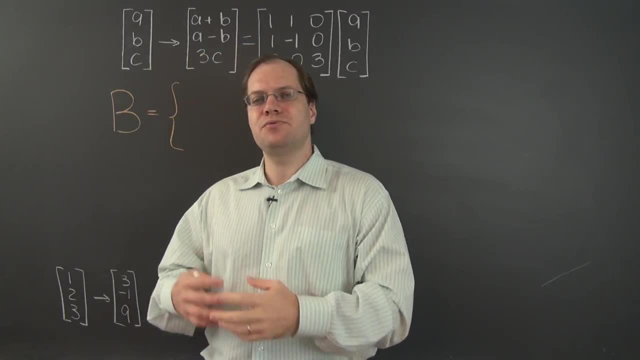 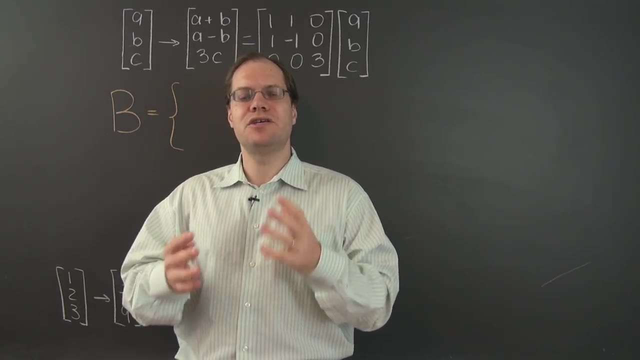 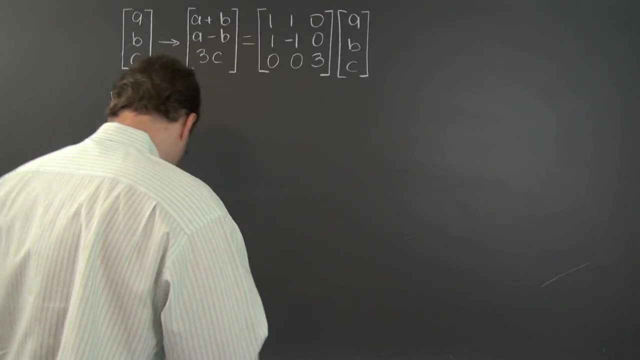 Represents this linear transformation in the component space with respect to this basis And, of course, it's going to be a different matrix, So it's very important to keep the two matrices straight. okay, now let's choose a basis and Compute the matrix. Here we go. I'll choose a basis That's not too simple, not too complicated. 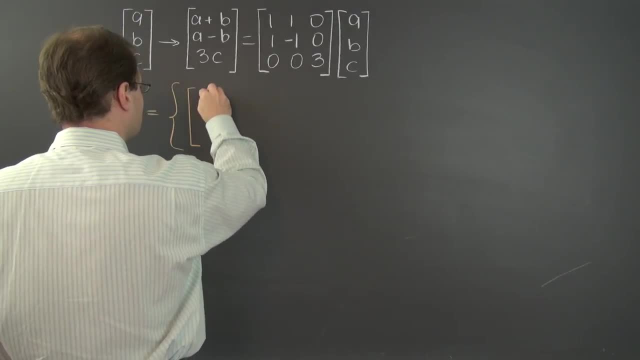 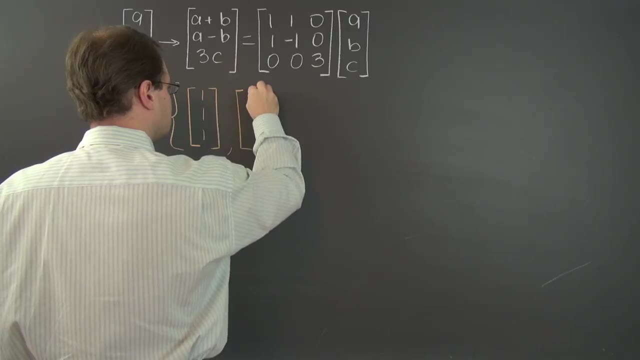 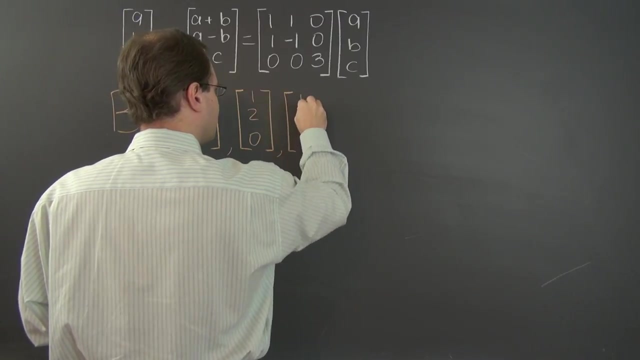 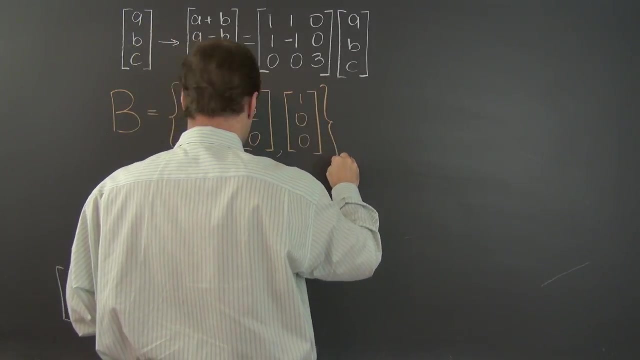 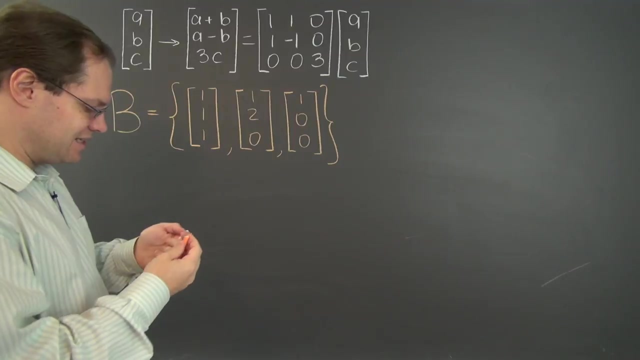 So how about we'll start with one one one, One, two zero And one zero zero, one zero zero. Okay, that's our first basis and that's the basis that will occupy this entire video. Okay, so let's begin constructing the matrix. Transformation needs a name. 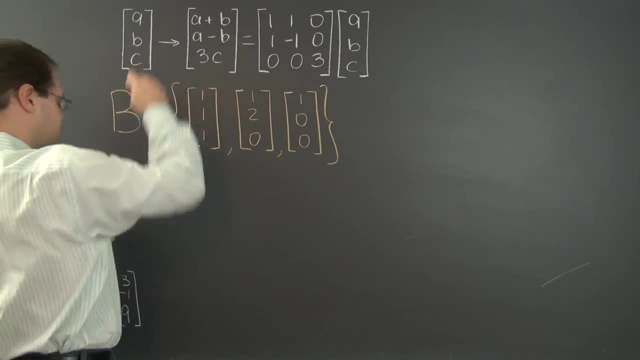 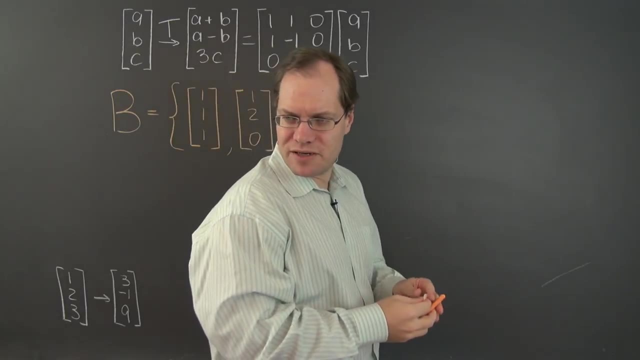 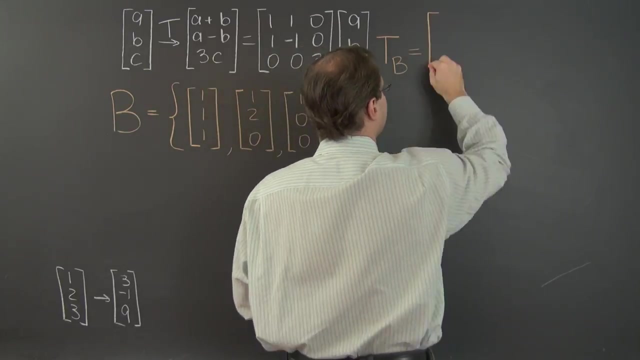 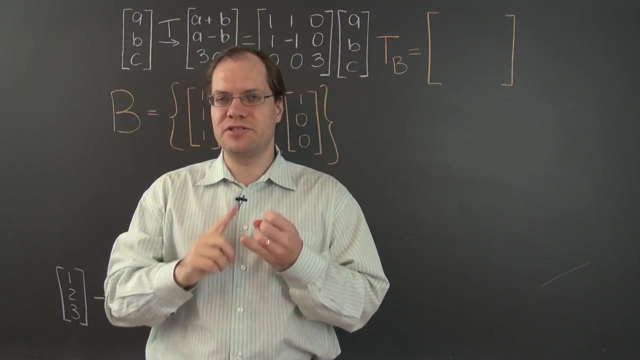 What's a good, good letter for it? I have a T, just for transformation. T and Here is T. Let me make sure we have space. we do right here. T with respect to the basis B. Okay, so the strategy is the same. we've already seen the strategy with geometric vectors and polynomials. 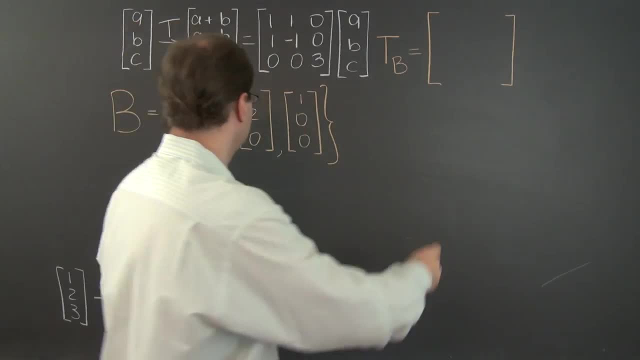 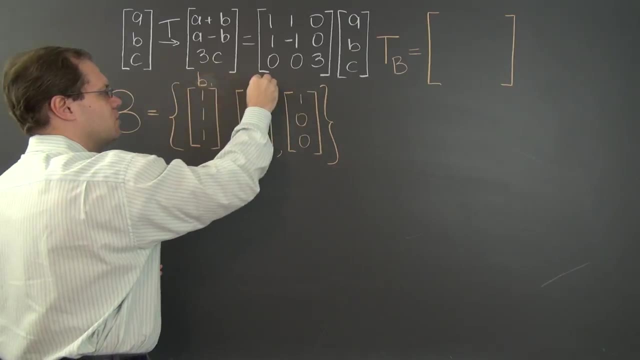 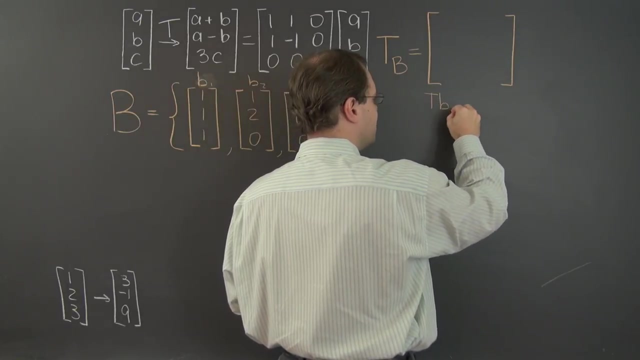 Now it's time to apply it to our end. So if we were to call these- well, that's actually called them something- e1. Well, the basis is called B, So why not be one B to be three, and of course, the first column will correspond to T of B one. 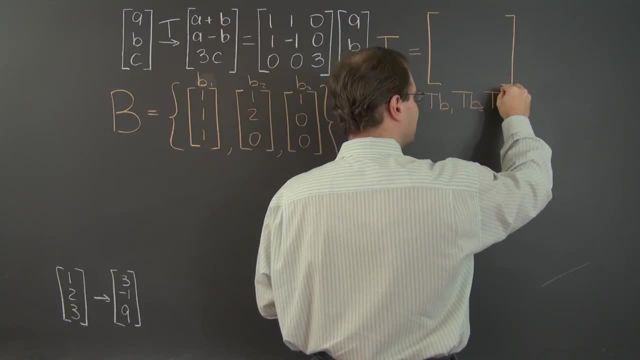 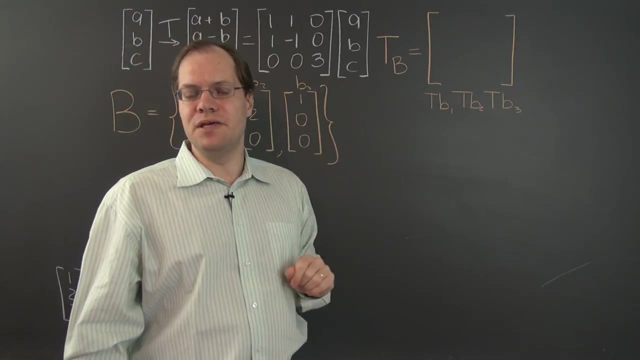 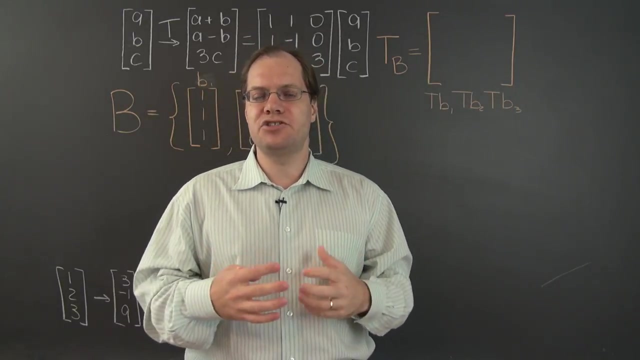 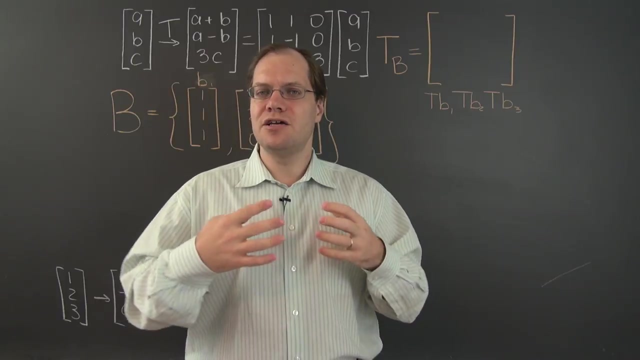 The second column will correspond to T of B two and the third column will correspond to T of B three. Let's figure out T of B one. That's how this matrix is absorbing the linear transformation: by applying the linear transformation directly- That's the only way at this point- to each of the basis elements and then capturing the result in terms of the coefficients. 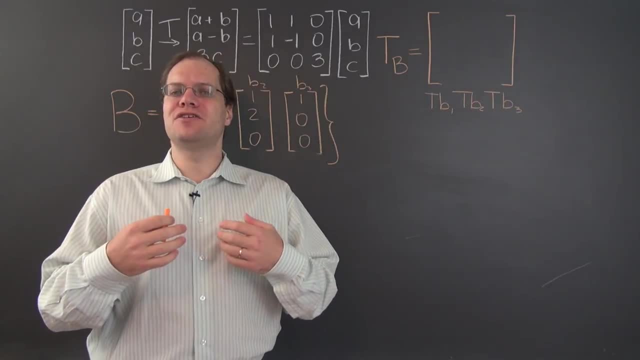 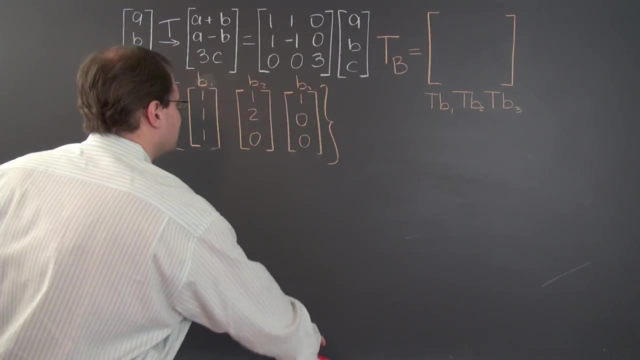 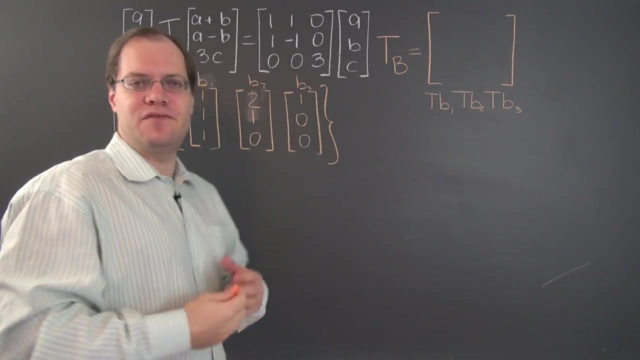 Actually, having worked through the whole example on camera, I realized that there are just too many fractions that distract from the main message of this video. So what I'm going to do is change the basis by switching this one and two And rerecord the second half of the video, So instead of the original basis that I just had on the board, 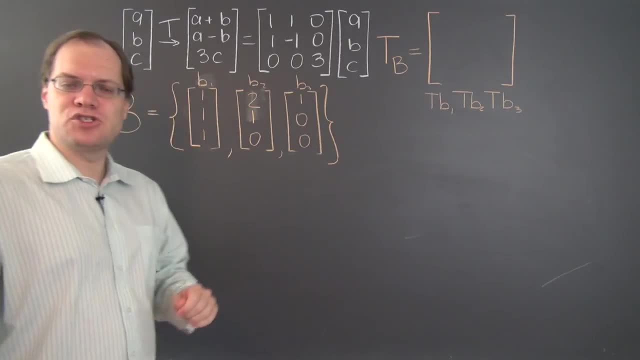 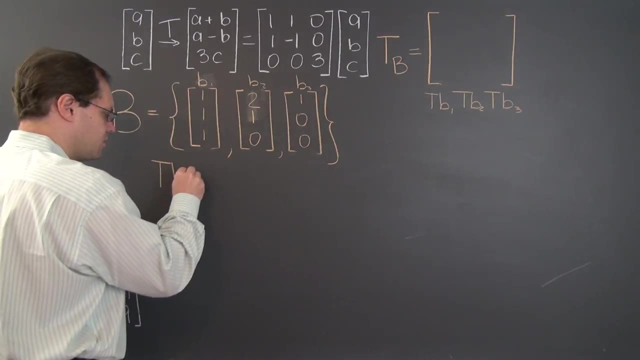 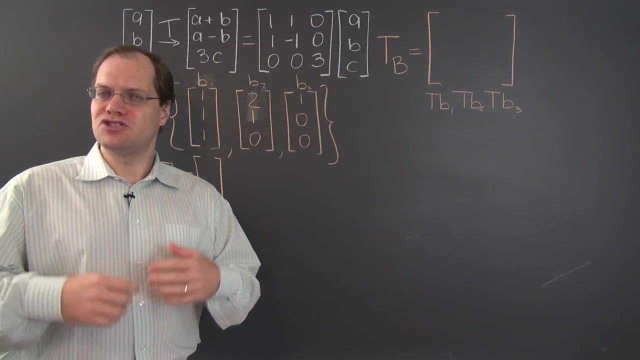 Let's work with this basis instead. So our first task is to figure out T of B one, so T of B one. We must apply this same transformation To the first basis element, just like we did in the case of geometric vectors and later polynomials, and the result is, of course: 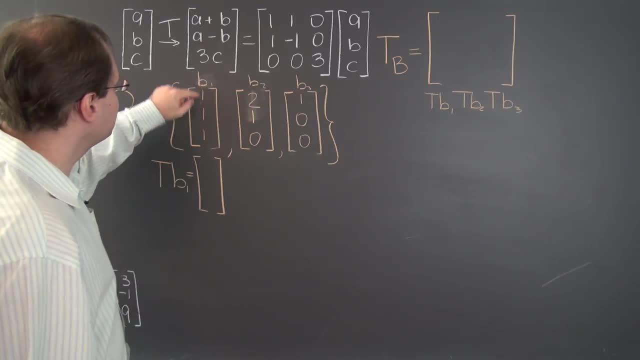 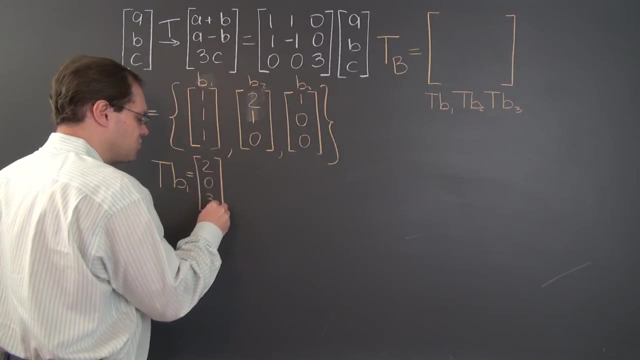 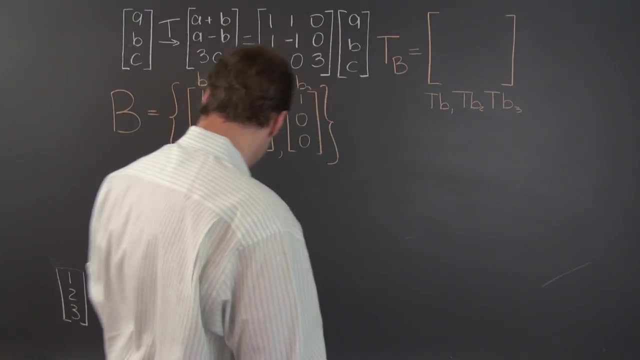 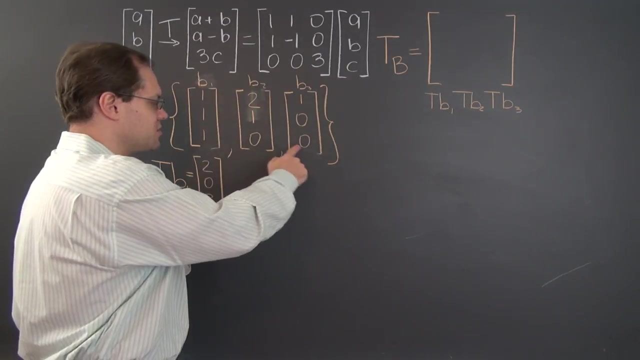 two zero three. Once again, the sum of the first two, two, their difference, zero, three times the last one. two zero three. and Importantly, it is not two zero three that goes as the first column here, It's not T of B one itself. What goes into the first column, it is its coefficients with respect to the same basis. 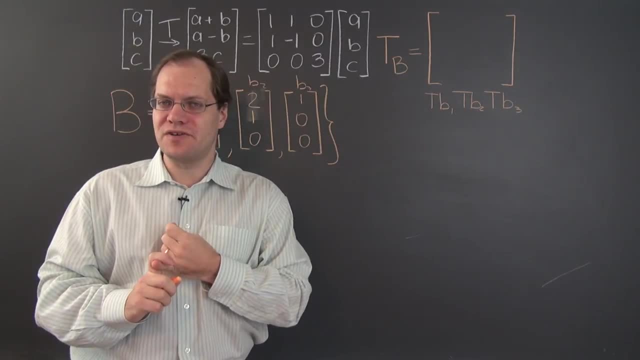 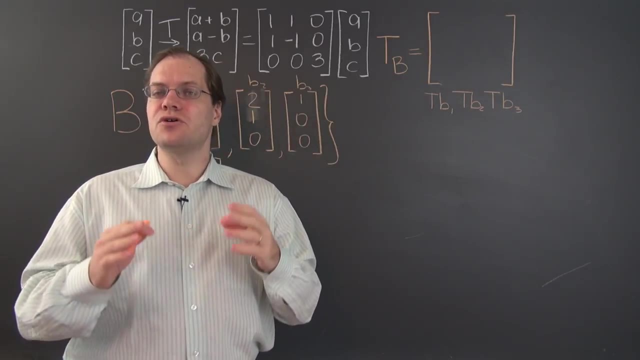 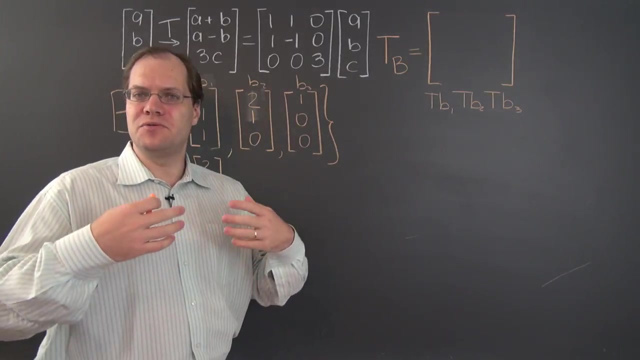 Now, this is the kind of mistake that we could not have made with geometric vectors And we could not have made with polynomials, but we can make rather easily with vectors from our end. So you have to be a little bit careful here. So it's not this vector, but instead following the pattern, as we did with other kinds of vectors. 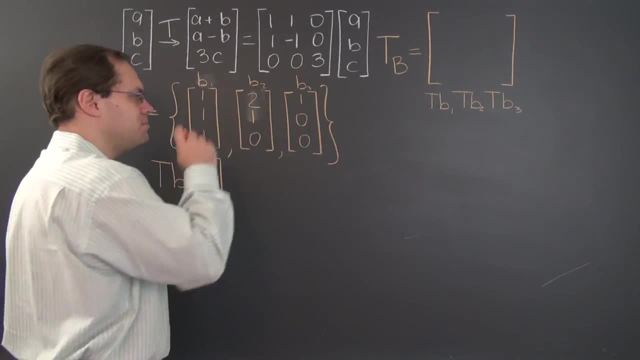 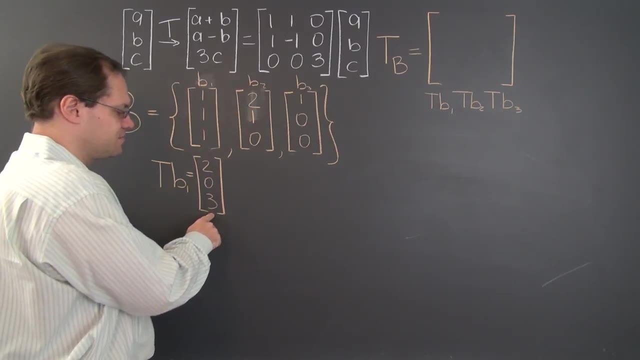 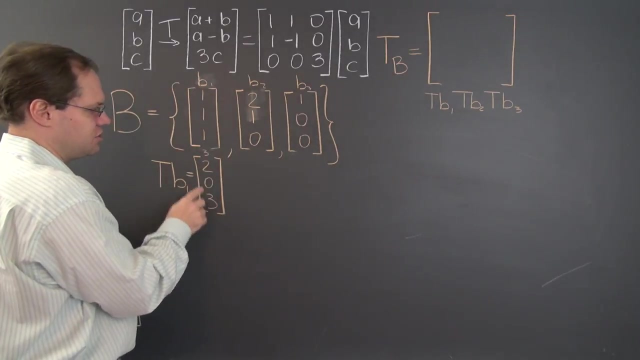 It is the components of T, of B, one with respect to the same basis That goes here as the first column of this matrix. So we have to decompose this vector with respect to this basis, and those Are of course three to get this. three. Here's our only chance, and once we have three here, we have to have minus three here. 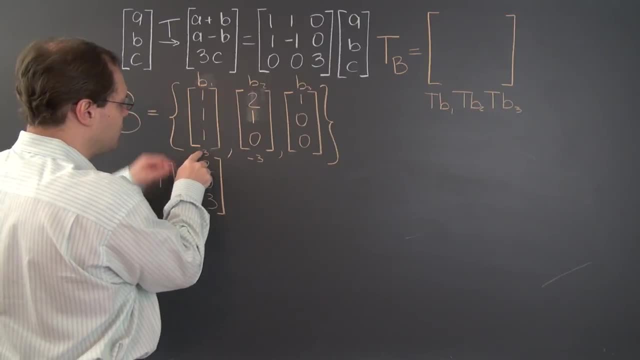 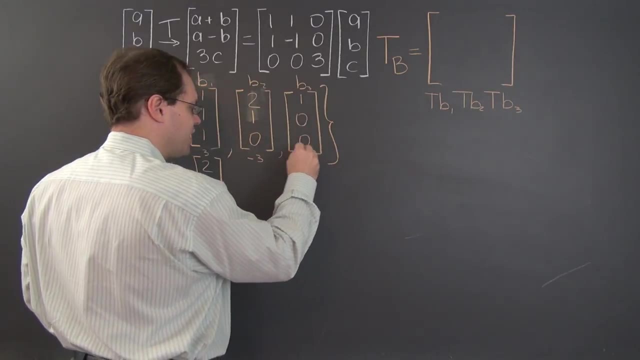 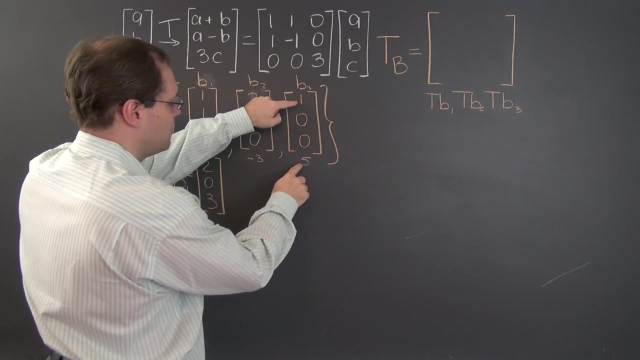 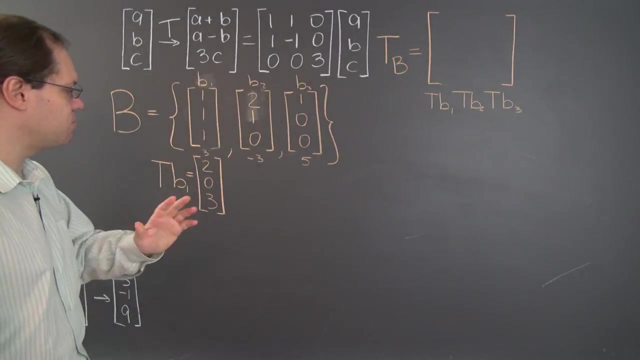 And then finally, to get this, two. so far we have three minus six minus three, so needs to be Five, let me just make sure. so in the first entry We'll have three minus six plus five, two, and the second entry We have three minus three, and in the last entry we have three. so perfect, so three. 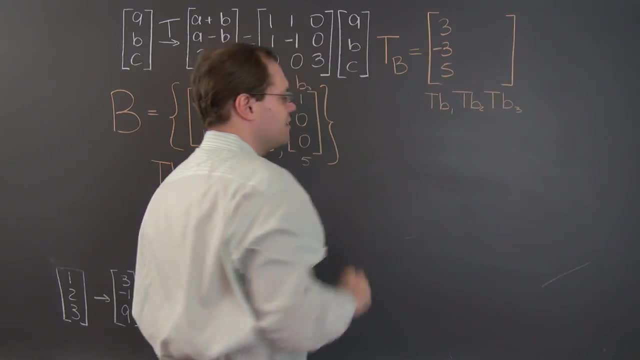 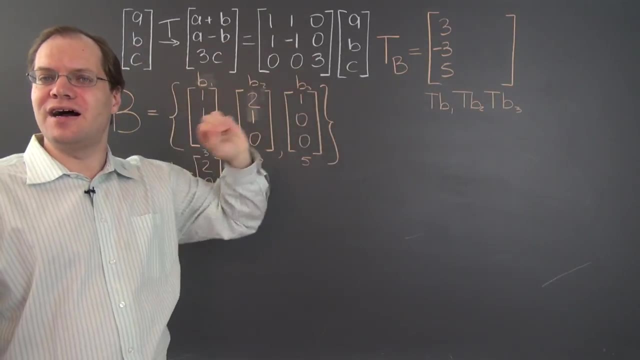 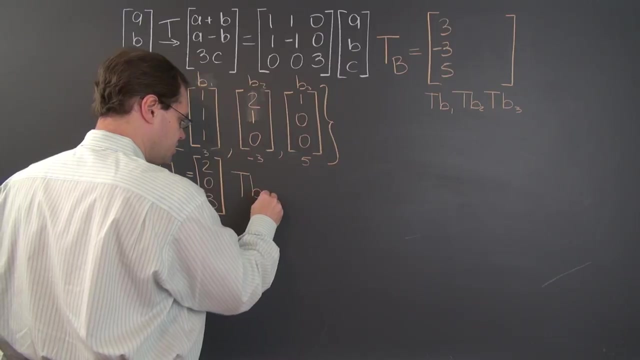 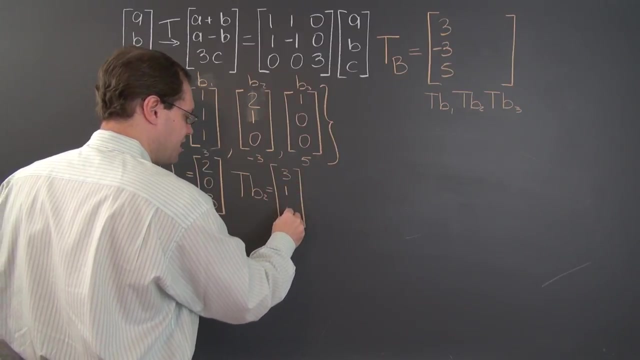 Negative three, Five. and you have to observe that the matrix that's emerging here is Completely different from the matrix that defines this transformation. Okay, next, T of B two. T of B two Is the sum of the first two elements. There are difference, and three times the last element. 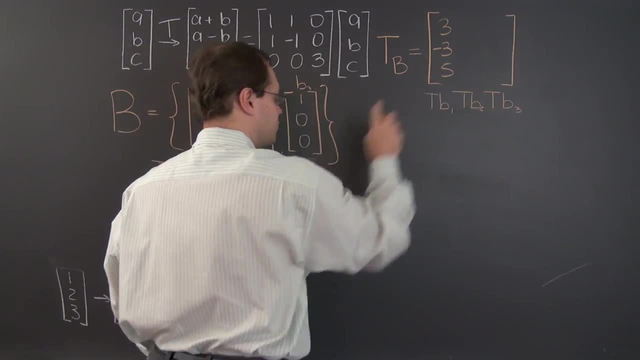 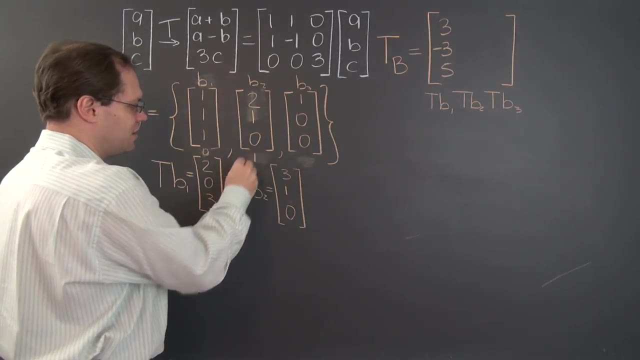 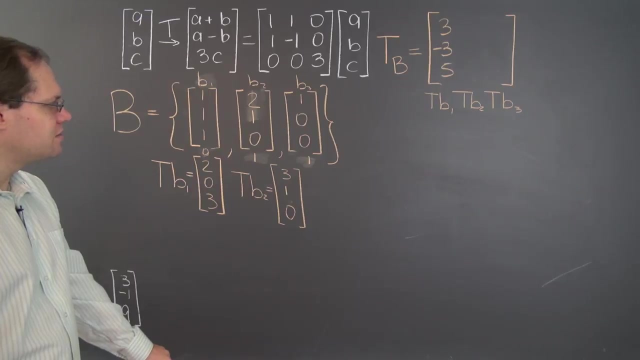 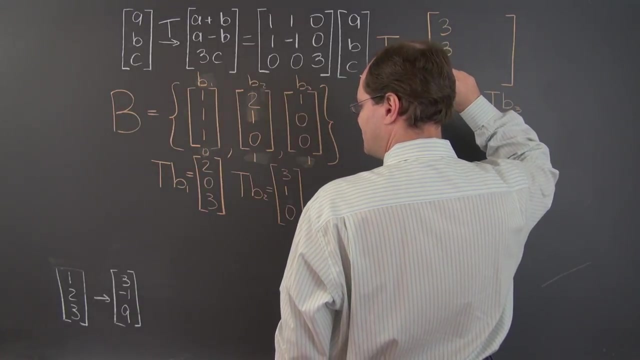 So, once again, it's not this vector that goes here, It is its components with respect to the same basis. so we have to take zero of this one, one of this one and one of this one. zero one one, Zero one one. all right, Just making sure one more time, Yeah. 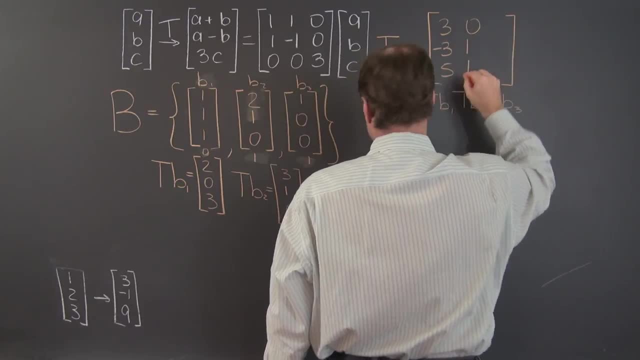 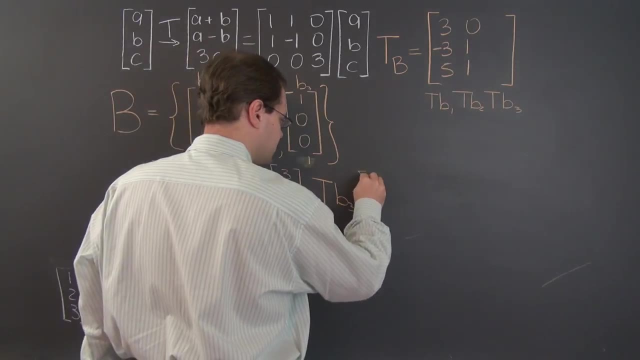 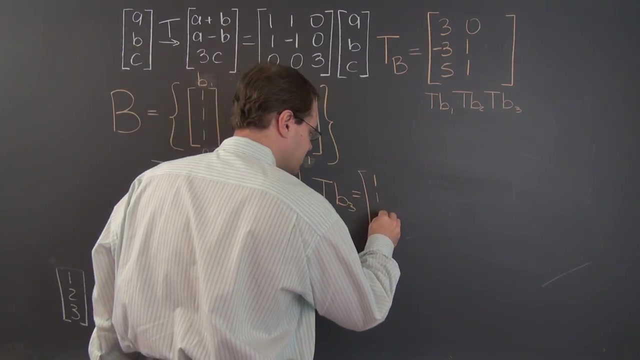 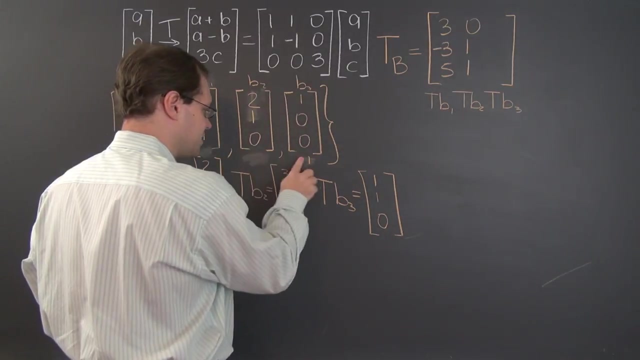 zero, One, one. and now for the last entry. T of B three equals The sum of the first two entries, their difference and Three times the last entry. Okay, and Decomposing this vector with respect to the same basis. We need none of this. one of this and more. 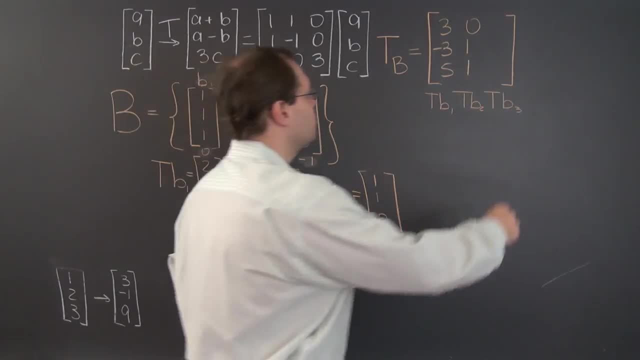 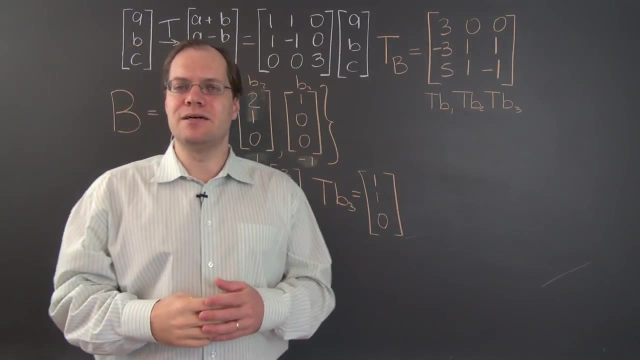 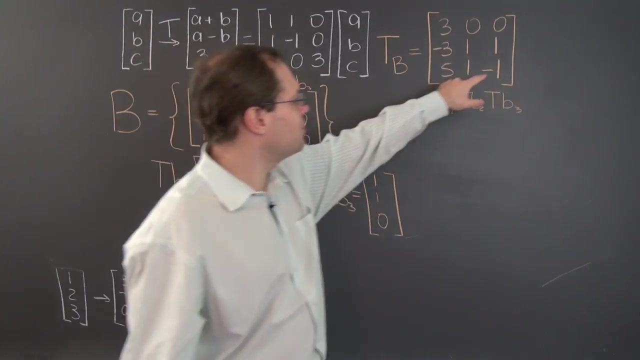 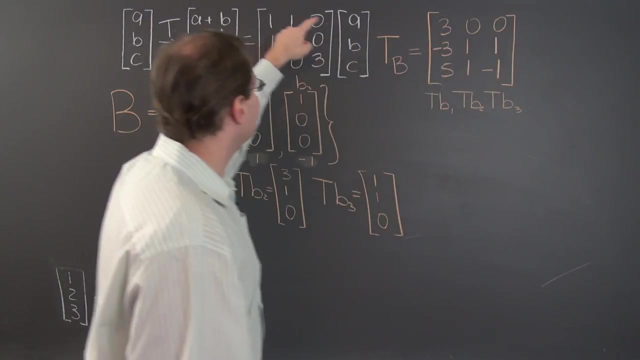 minus one of this, That's right. zero one, zero one, negative one, and We're completely done. So a couple things to observe. number one: This matrix is completely different from this matrix, even though unexpectedly and Surprisingly total coincidence, I believe this section is kind of reminiscent of this one. but that's just one little feature. 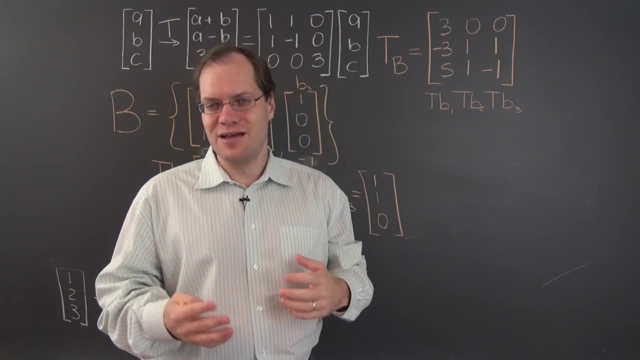 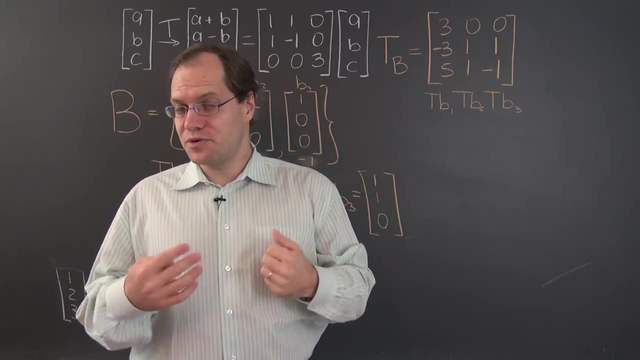 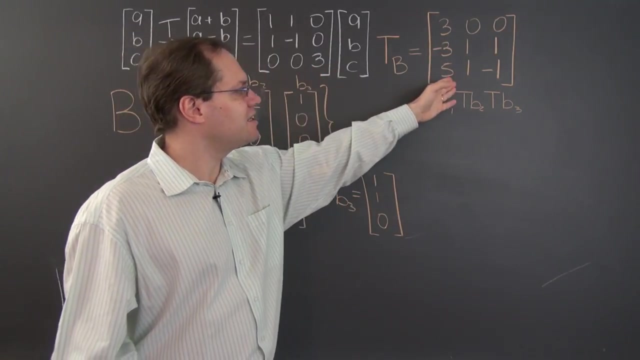 Overall, this matrix is completely different and then we chose in another basis, We would get an altogether different matrix. so different bases, as we've already realized, lead to different matrices and, Of course, the point that I was actually making is that this matrix that represents this linear transformation in the component space with respect to some 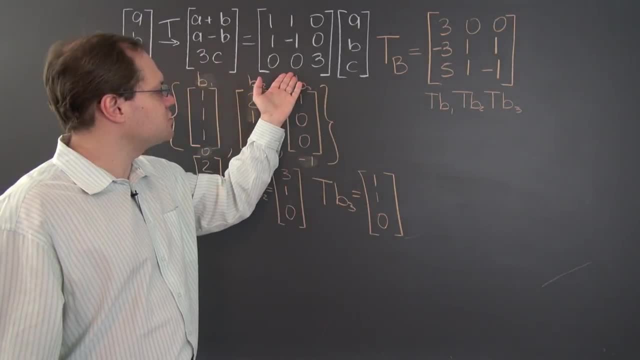 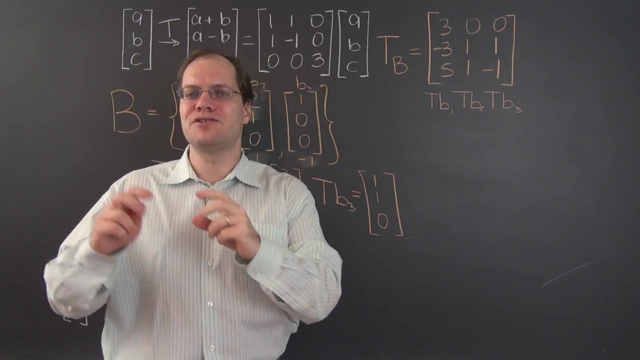 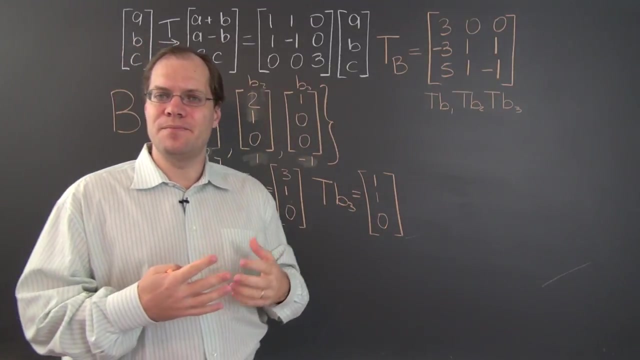 Basis is completely different from the matrix that defines it in the real world space of our end. So a little bit confusing because of the real world- and you see the air quotes, the quote-unquote. real world Looks exactly the same, as the exact same kinds of vectors, as the components base. 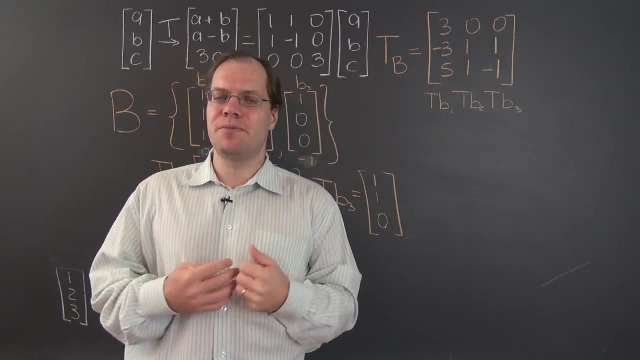 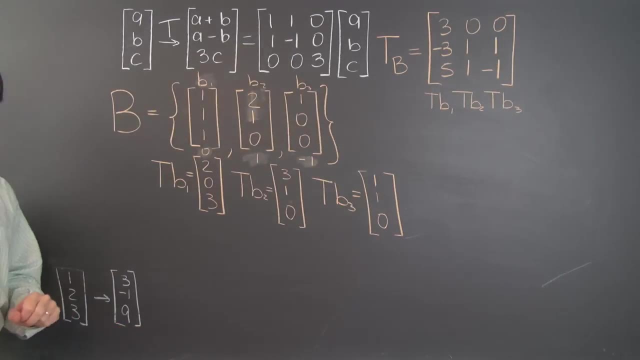 That's that special feature of our end that just calls upon us to be a little bit careful. So, as the final thing, let's just make sure that one, two, three, had we gone through the component space, would also result in three negative one, nine. So once again making sure. 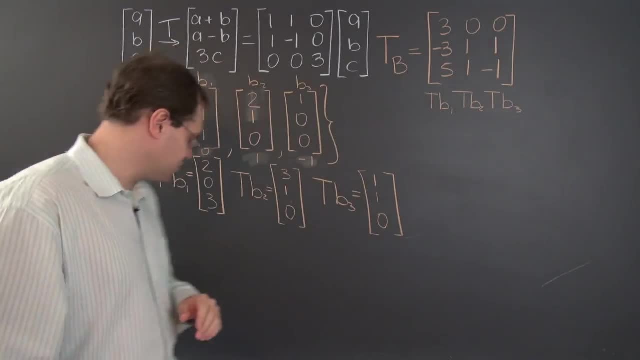 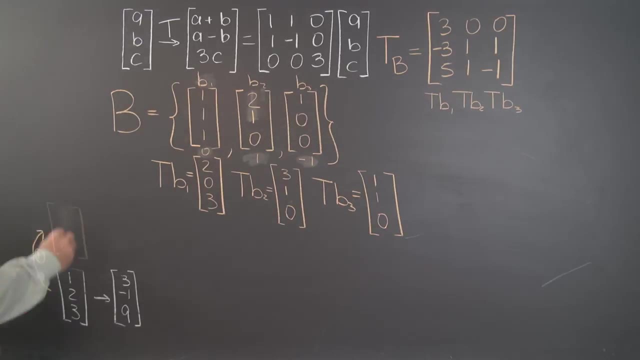 sure that our overall strategy works, Not so difficult. First step, number one: decomposing with respect to the basis. So to decompose one, two, three, we must have three of this basis element to guarantee this last three, Now that we have three. 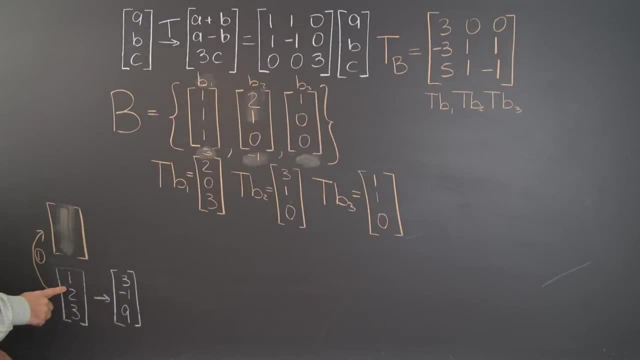 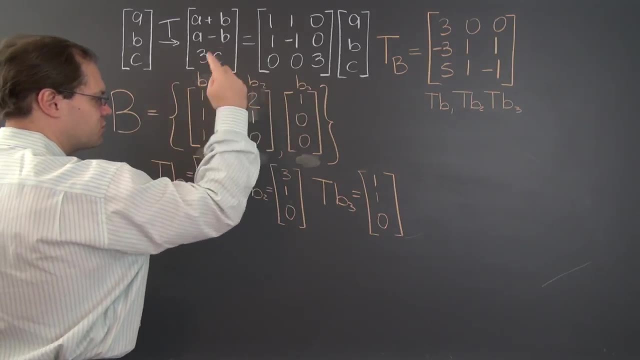 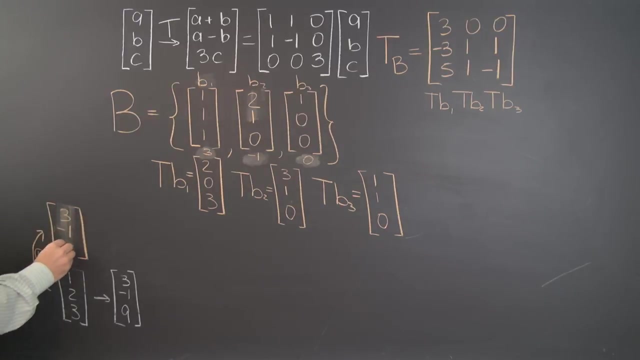 here. we need minus one of this one, so that the second entry is two and we need one in the first entry. Three minus two One. we already have one in the first entry, so zero of the last one. So three negative one: zero. Three negative one: zero. 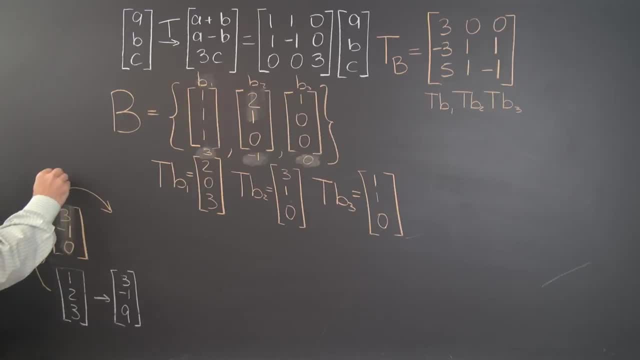 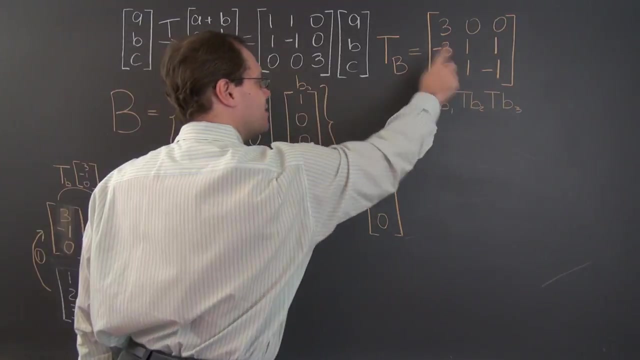 Now step number two. we need to multiply this vector of components by the matrix T, sub B, times three negative one, zero, And the result would be- let me put sub B here to make sure that these are the components of this vector with respect to the basis B. So now multiplying this. 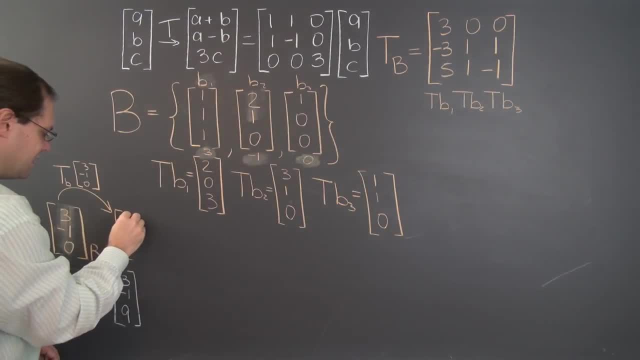 matrix by this vector gives us nine and minus nine minus one, minus negative ten and finally fifteen minus one. ok, and the final step is to translate this vector that's given in the component space back to reality. So we have to take nine, of this one negative. 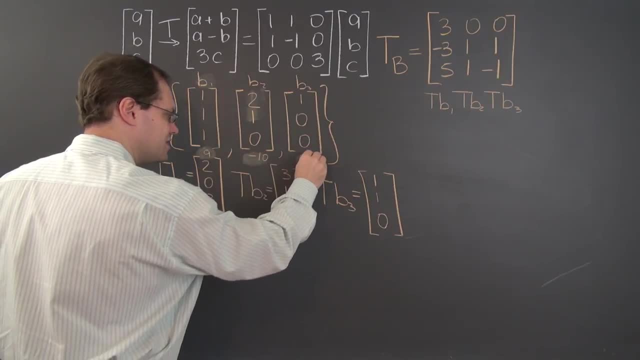 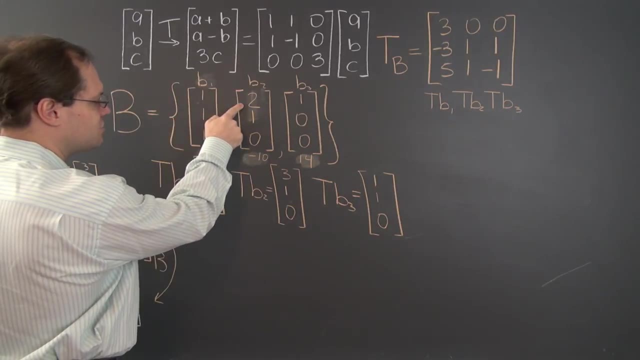 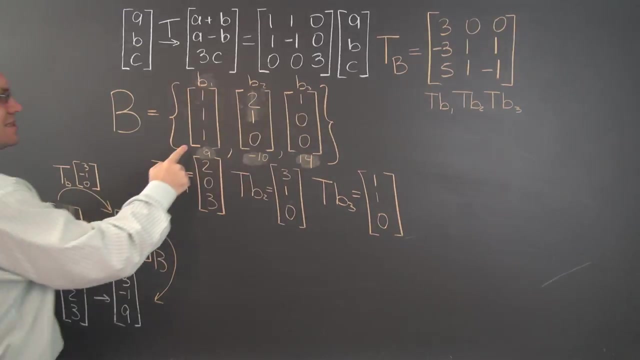 10 of this one and 14 of this one. This is the synthesizing step and let's see what we get. in the first entry, We get 9 minus 20.. That nine minus twenty is mine: 11 plus 14- 3. in the second entry, we get 9 minus 10 minus 1. and in the last entry, 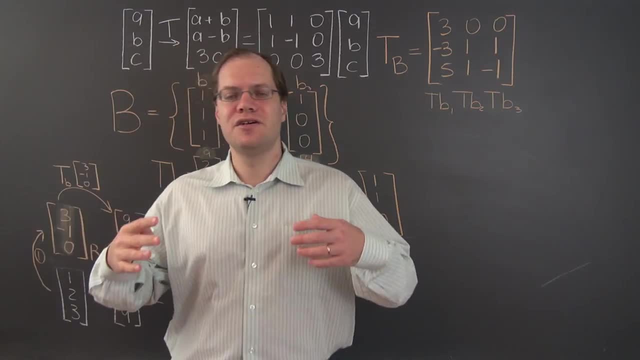 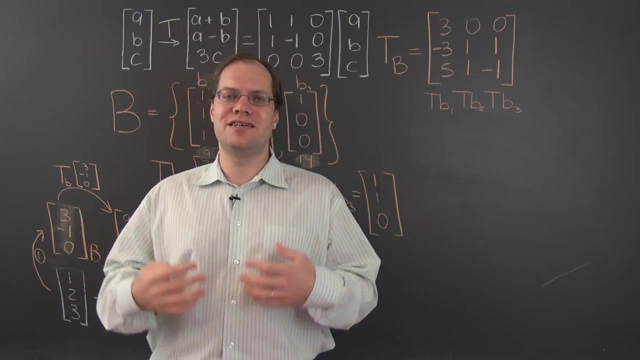 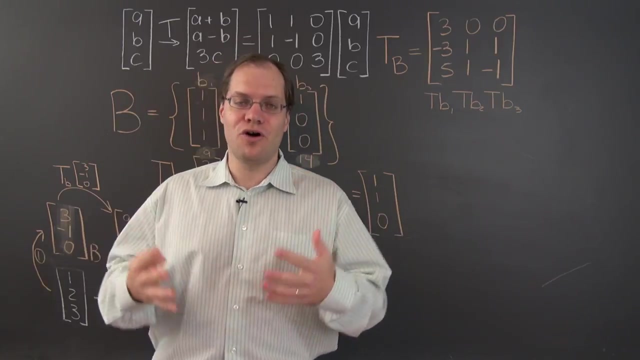 we have 9, so it works just as well as it did in the first two kinds of spaces that we consider: geometric vectors and polynomials. and of course, we're seeing over and over again that this strategy works in all spaces with respect to, for all linear transformations, with respect to any basis. it's a very general and 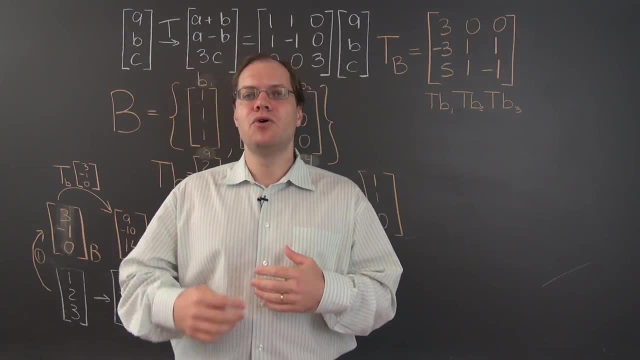 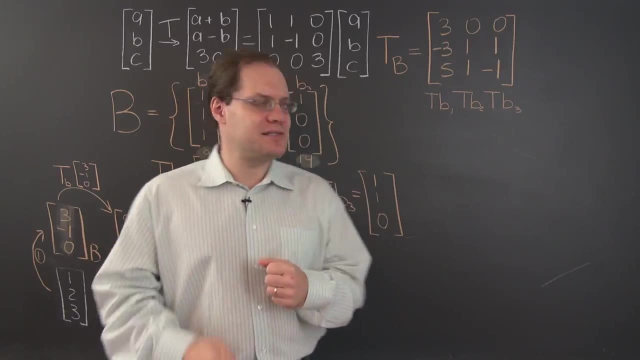 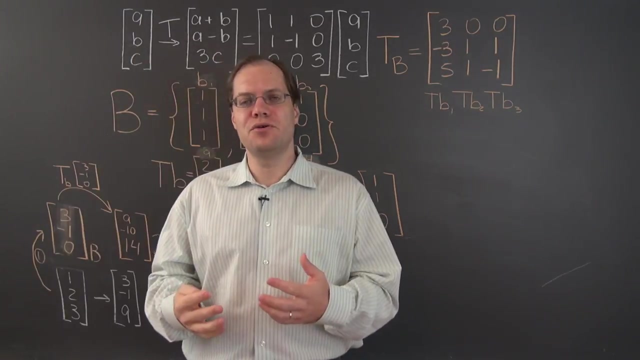 robust strategy. so we're done with this example. what we're going to do next is consider this standard basis in R3. the standard basis in R3 is 1 0 0 0. 1 0 0 0 1. so before you watch that video, why don't you try and work out the same? 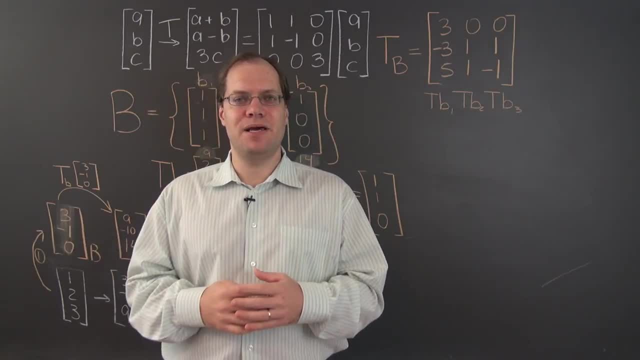 example, same linear transformation, but with the standard basis in R3.. you.